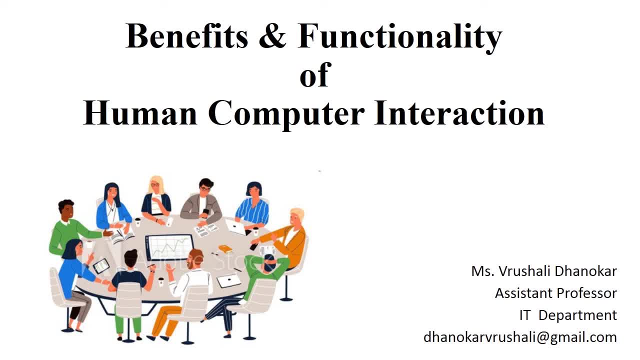 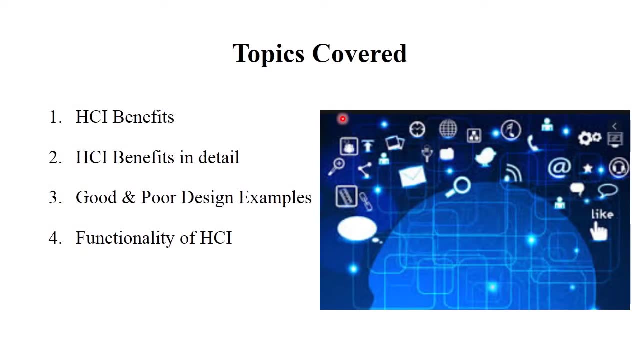 every organization. Human-computer interaction is beneficial, Right? So let's see the exact benefits and functionality of human-computer interaction, Okay, Next. So in this video, the below topics are covered. The topics includes HCI benefits, HCI benefits in detail, good and poor design examples and functionality of HCI. Okay, So let's see human-computer interaction benefits. 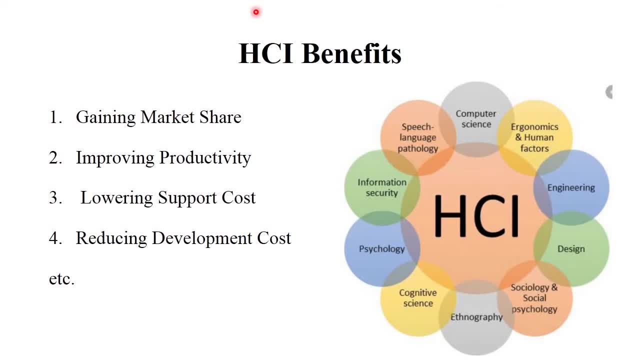 Okay. Next See: human-computer interaction have benefits in each and every organization and each and every field. Right Human-computer interaction can be used in computer science, ergonomics, engineering, design, then sociology and social psychology, ethnography, cognitive science, psychology, information security, speech, language pathology and computer science department. Okay. 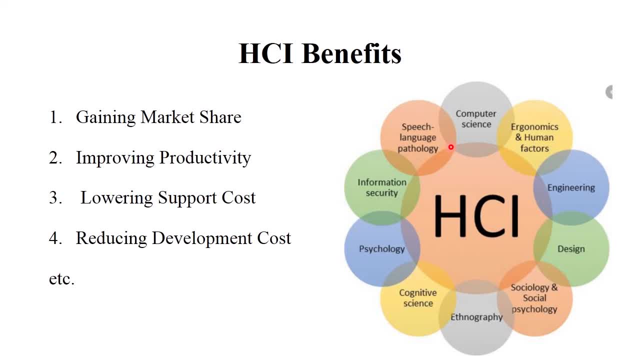 It means that each and every organization, each and every field institute, human-computer interaction is used. Okay, So obvious it has benefits for from them, Right? So main benefits of human-computer interaction is gaining market share, improving productivity, lowering support cost and reducing development cost. Okay, These are the some main benefits of human-computer interaction. So let's see one by one. 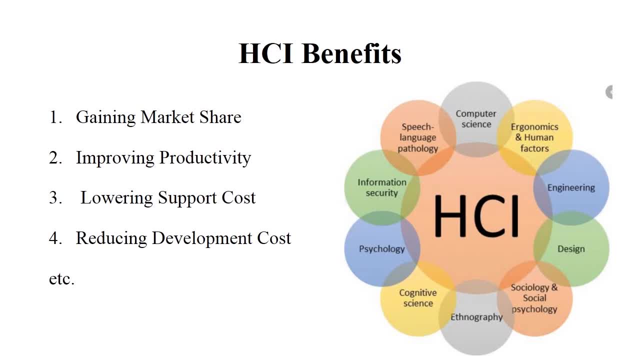 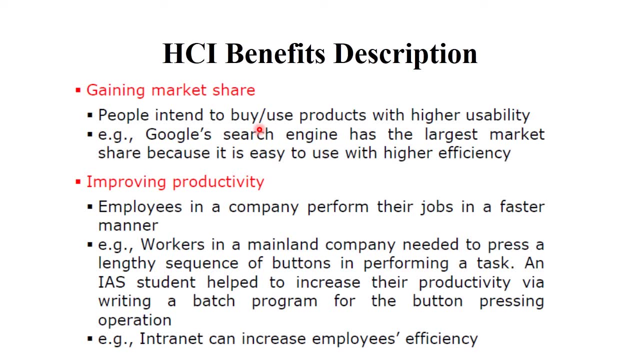 Exactly These benefits are given. Okay, Next, Now see here the benefits of human-computer interaction in more descriptive way. Okay, The first benefit is gaining market share. Okay, People intend to buy and use products with higher usability, Right. For example, Google search engine. Google search engine has the largest market share because it is easy to use, with higher efficiency, Right? So let's see one by one: 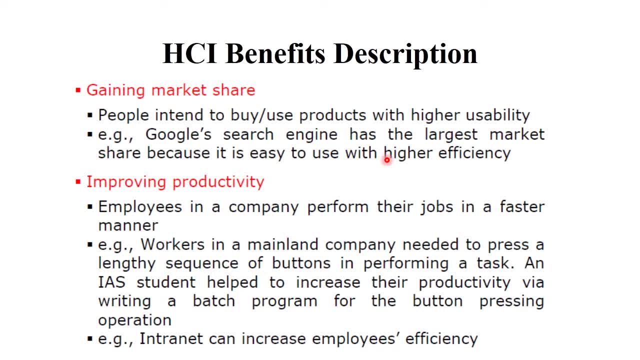 Exactly, Other than google search engine, there is Opera, Yahoo. This kind of engine also available, Right? But google search engine has the largest market or it has higher efficiency because it's easy to use and easy to learn, Right? So this is benefit of gaining market share. is the benefit of HCI, Clear, Okay? The next benefit is improving productivity. Employee in a company perform their job with higher productivity, Right? So these are the main benefits of human-computer interaction. So let's see one by one. 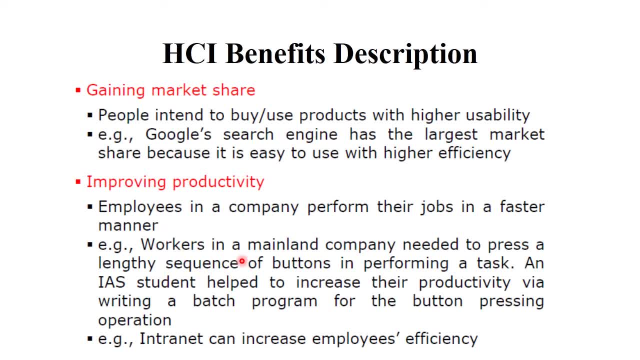 in faster manner. Right, For example. workers in mainland company needed to press a lengthy sequence of buttons in performing a task. An IAS student helped to increase their productivity via writing a batch program for the button pressing operation. Right, For example, when you press a particular button for each and every action is performed. 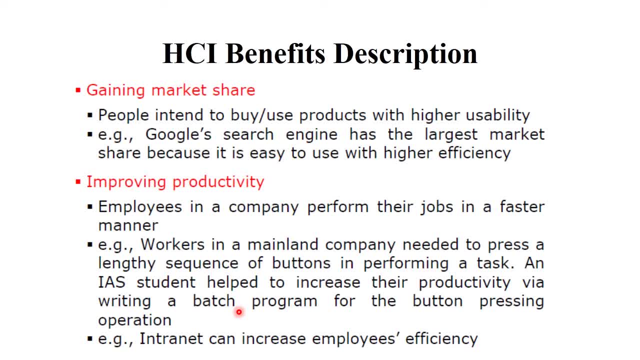 Right, And from that you have to use batch of operations. Ok, So multi-grading, multi-tasking- this kind of concept is used for improving productivity. Ok, Means in minimum time you have to implement the particular product and it gives the output in minimum time. Right. 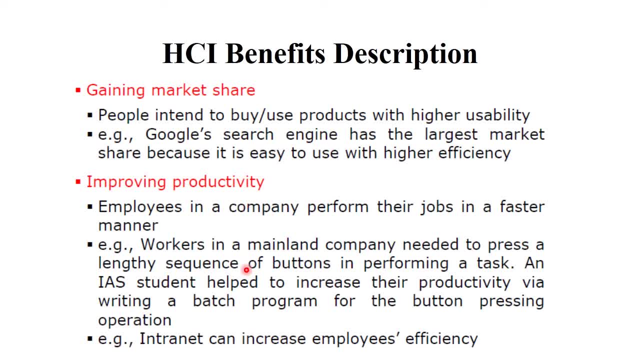 Which is called as improving productivity, And internet can also increase employees efficiency. Clear Internet provide each and every output in more quick way or in the within a second Right, So this is called as improving productivity. Ok, So improving productivity means to performing operations more fast, Multi-grading or multi-tasking. 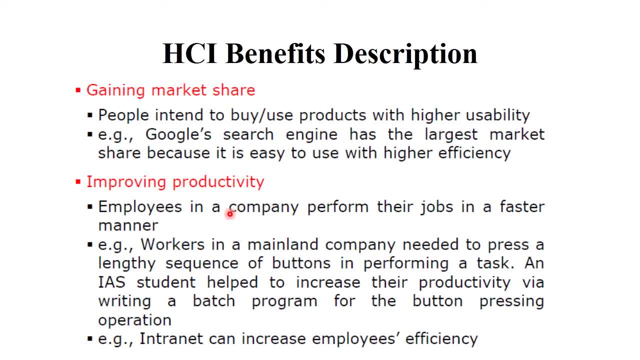 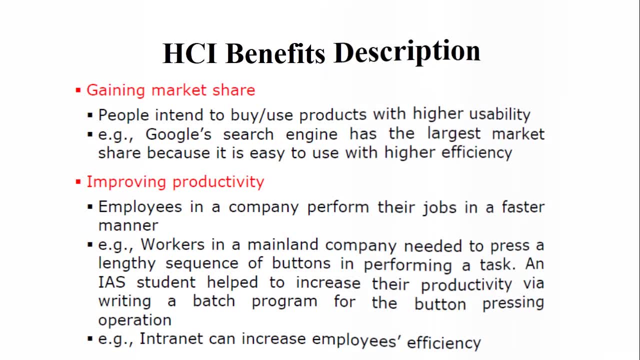 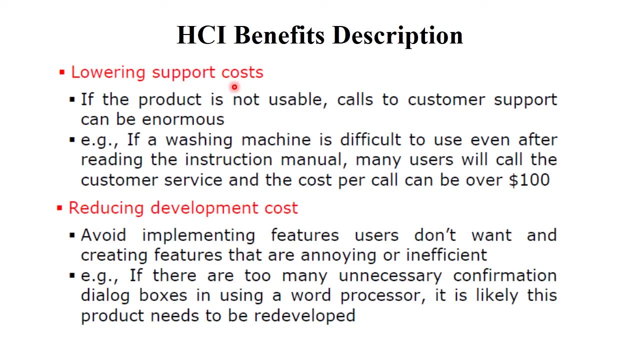 this type of concept is used for improving productivity, Clear. So these are the benefits of human-computer interaction, Ok. Next. So next benefit of human-computer interaction is lowering support cost. Ok, If the product is not usable, it calls the customer support. 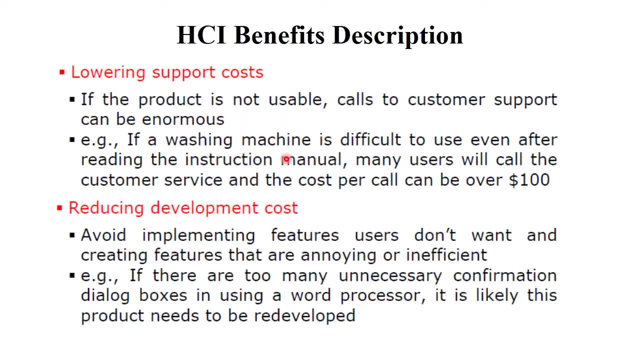 can be enormous. Ok, For example, if a washing machine is difficult to use even after reading the instruction manual, So many users will call the customer service and the cost per call can be over dollar hundred rupees. Right, So it is a benefit of human-computer interaction. You have to. 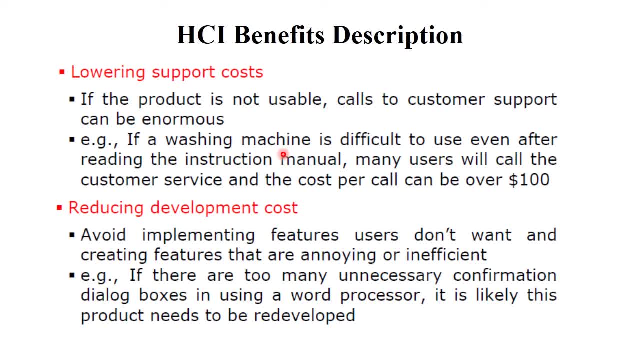 make such type of model where no need of customer services Right. So by using, by reading the instructions of manual, user can use the particular product. This is the more beneficial benefit of human-computer interaction. Ok, So by using, by reading the instructions. 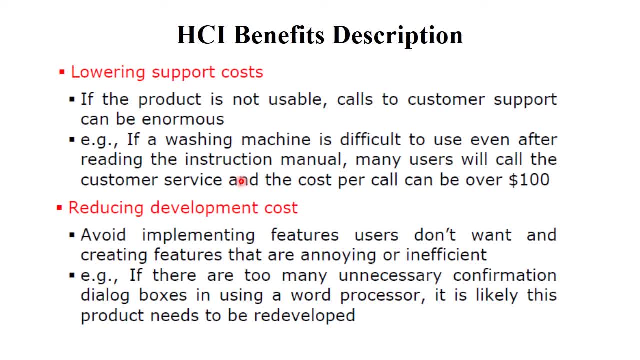 of manual, user can use the particular product. This is the more beneficial benefit. Ok, So way clear. ok, the next benefit of human computer interaction is reducing the development cost. ok, so avoid implementing features user don't want and creating features that are annoying or efficient. ok, you have to develop a. 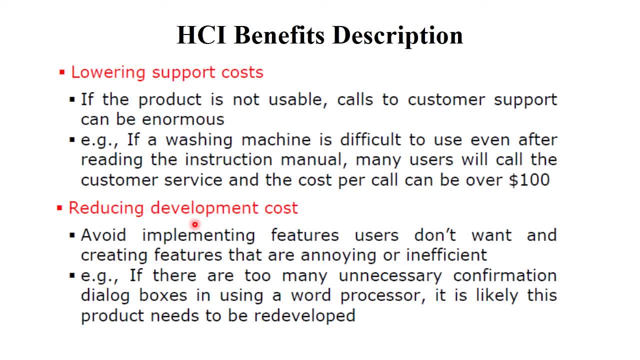 particular product which have more easy features, not annoying or any inefficient features. ok, for example, if there are too many unnecessary confirmation dialogue boxes is using in word processor, it is likely to this product need to be redeveloped. right, you have to use Microsoft Word or you have, you will also. 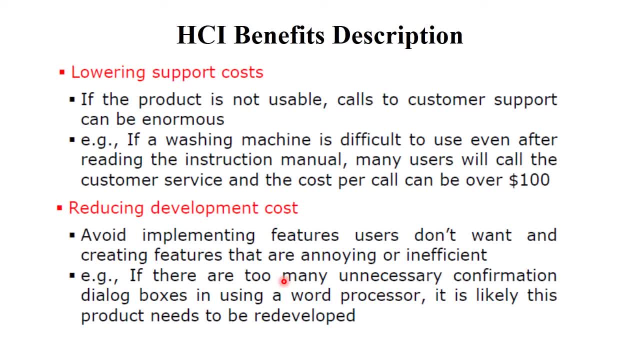 used a different types of application like whatsapp, facebook, insta, so this all type of operation is very easy to use. you can easily post a photos, you can easily upload the videos, right? you can easily send a friend request to another other one, right? so this all type of applications is very easy to use and easy to learn, right? so it also 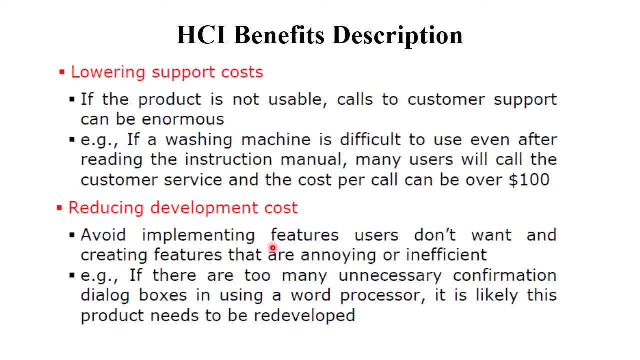 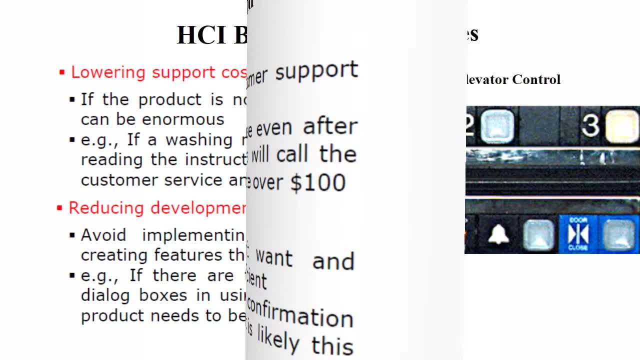 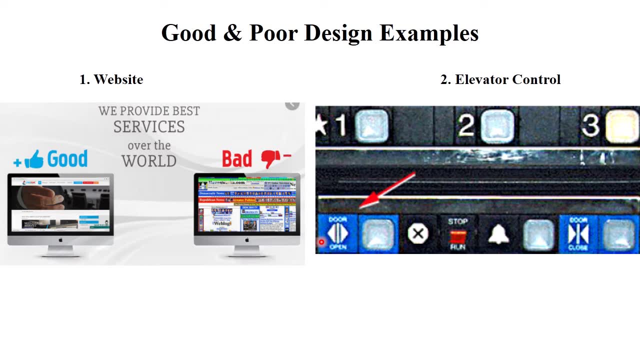 reduced the development cost. clear. so this is the benefits of human-computer interaction, right, clear, ok. next, there are some good and poor design examples. ok, human-computer interaction always support only good design examples, because this good design examples are beneficial For each and everyone, And good design examples include: 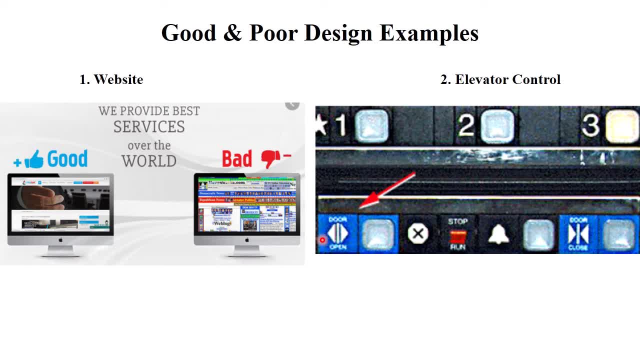 Usability, And usability means Easy to use And easy to learn, Clear, Ok. Now see here, in this first example, This is the example of website. So there are two computers Right. So in this computers The user interface website Is very, Very good to arrange. Ok, Each and everyone is arranged. 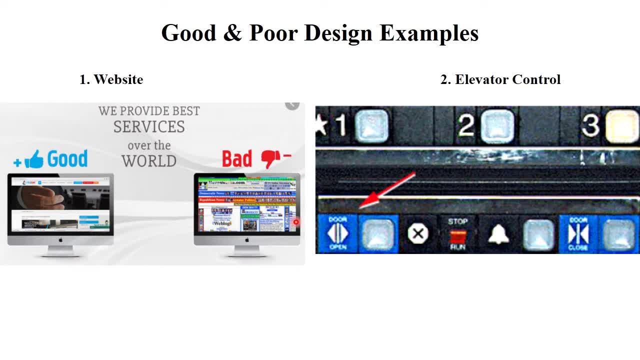 In more, More good way, Ok, But in this website There is very collapse For each and everyone use. Ok, It Don't easy or difficult to find Each and everything Clear. So this is a good design And this is a bad design. Ok, The format of this website is good. 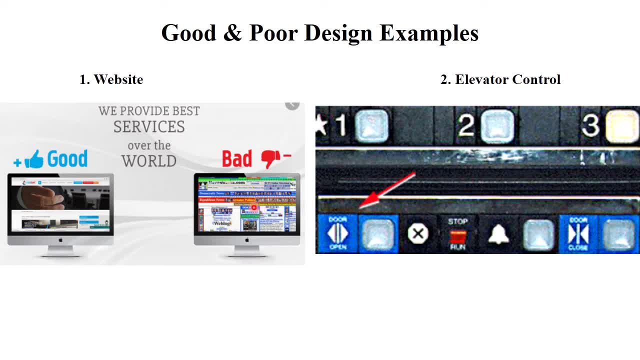 The format of this website is bad, Clear. So this is the example of good And bad websites- Clear. Next, Again Another example of elevator control. In this elevator control, All these buttons Like buttons One, Button Two And button Three, All are like same way. Ok, It doesn't provide any differential. 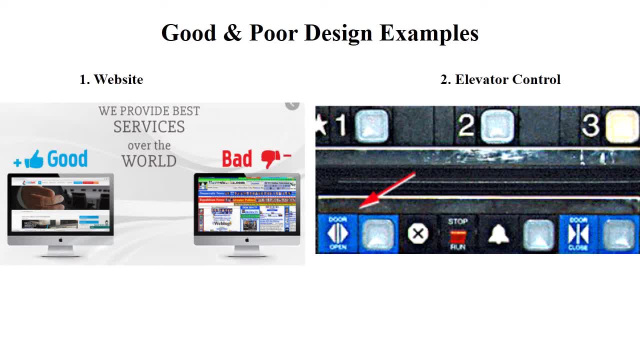 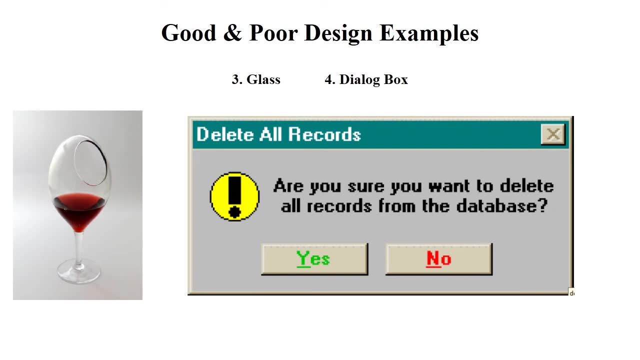 So user gets confused Which types of buttons works in which way. Clear. So this is a bad design of elevator control. Clear. So this is the example of good and poor design. Clear. Ok, Next, See here. This is another example of good and poor design. See here In third example. 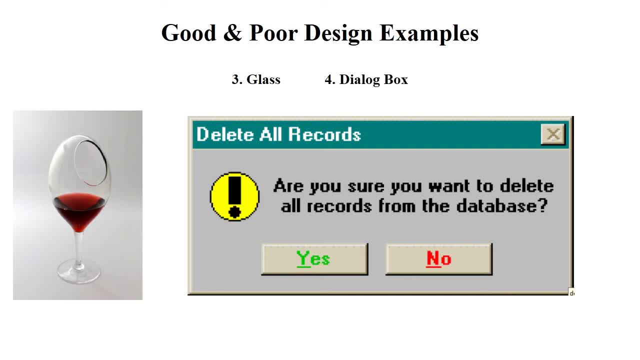 There is glass. Ok, Now how to drink by using this glass? This is not possible, Right? So this is a poor design example, Clear, And another example is dialogue box. Dialogue box shows notification Write, delete all records And also show the message or error, That is, are you sure you want to delete all records from the database? 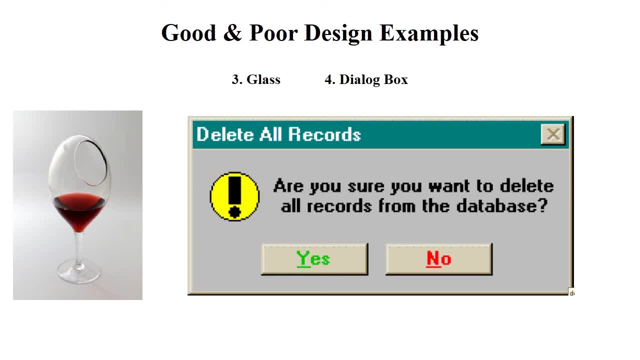 And also given two options. That is yes or no. It is a clear design. User does not get confused By seeing this dialogue box. Clear, So this is a bad design And this is a good design. Clear, So this is all about good and poor design examples. Next, Now see here: 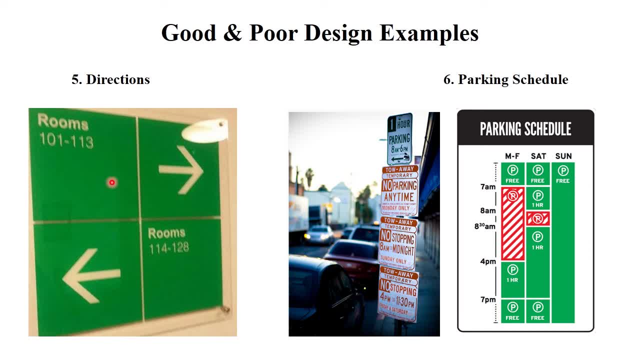 In this example. This is a direction example. Ok, This direction And this is a left and right directions. Right And rooms numbers are given, But Customers may get confused Whether this arrow is related to this Or whether this arrow is related to this. Is this good design? No, This is a poor design. 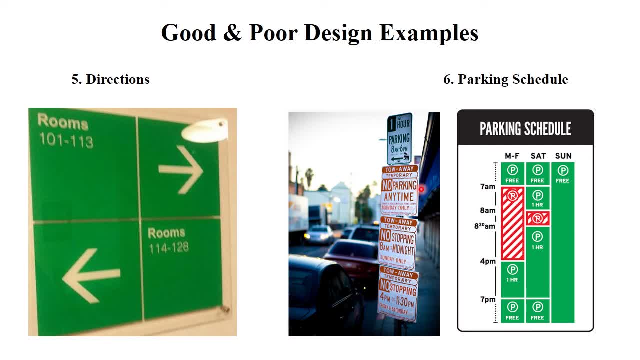 Clear, Ok, Ok. The another example is this: This is a parking schedule. Ok, In the first First board It may be written as: One hour parking, 8 am to 6 pm, Right? The next one is right: No parking anytime. Also, this show another information, So Customers get confused. 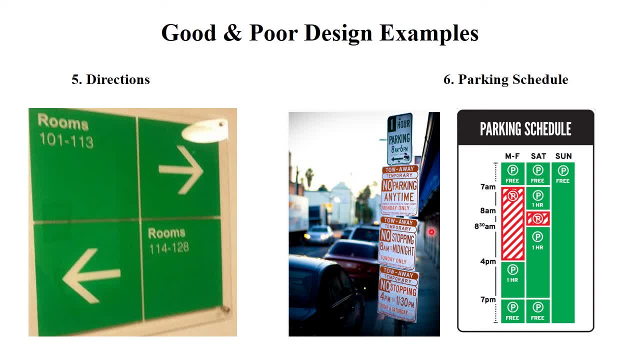 What exactly means that? Ok, So this is a poor design, Clear, So this design convert into this format: This is a parking schedule. Ok, This is 7 am slot And this is 7 to 4 am slot And 4 to 7 pm slot. Clear, So this parking schedule design is more corrective way. 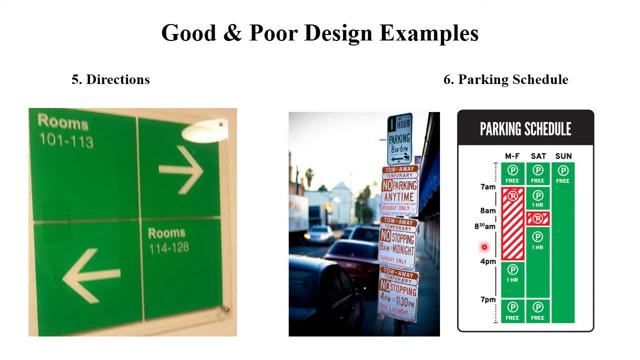 Right User gets understand in more easily. Clear So this is a good design example. Clear So this is good and poor design examples. So when you will implement a particular product, You have to focus on that thing. Your website, Your product Is very easy to use, Easy to learn. 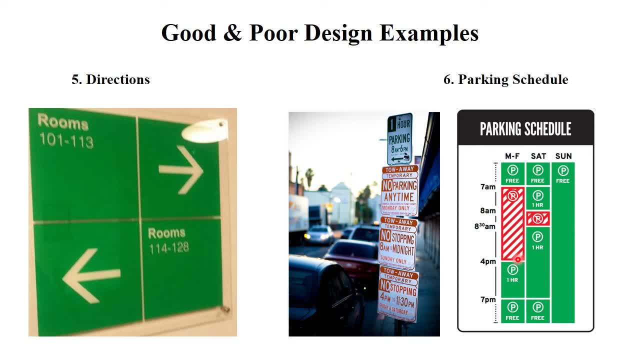 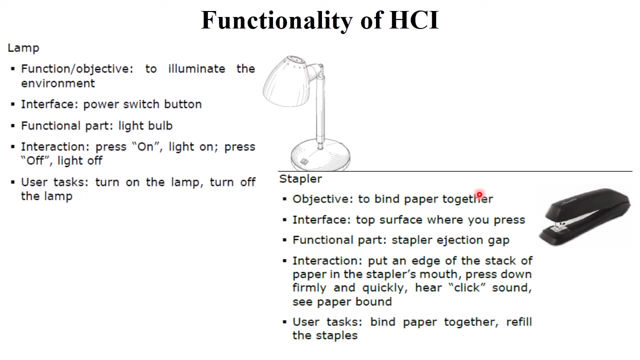 And always use good design. No, any complicated formats in that. Clear. So this is a example of good and poor design. And human computer interaction supports all the good designs. Clear Ok Next. So this is a good design example. Clear Next, The functionality of human computer interaction: See here. 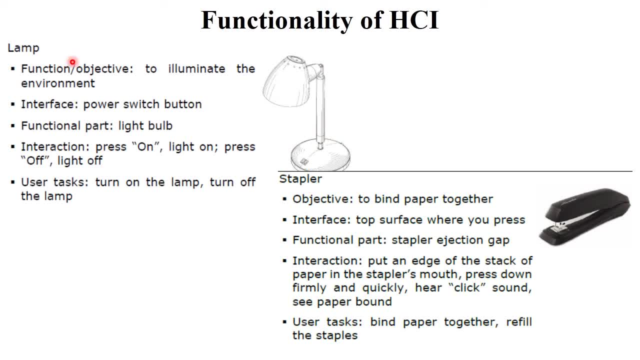 This is a example of lamp. Ok, There are a total 5 options are given Functions, Interface, Functional part, Interaction And user task Clear Now see The function and objective of lamp is To illuminate the environment. Right Interface is power switch button. Functional part is light bulb- Ok, Interaction is: 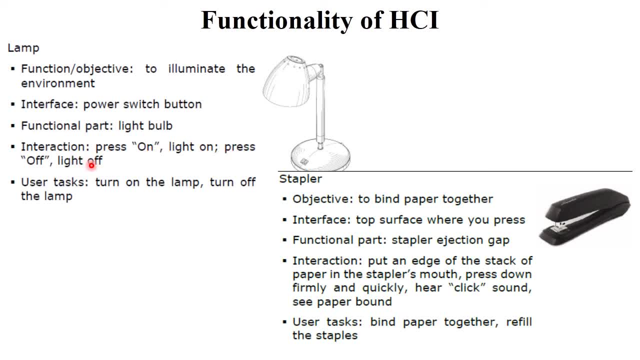 Press on Light on, Press off Light off, Clear, And user task is: Turn on the lamp, Turn off the lamp, Clear. So each and everything is clear In this way, Right, So you have to develop. the product Is more usable And more clear, Clear. Next thing, there is stapler. 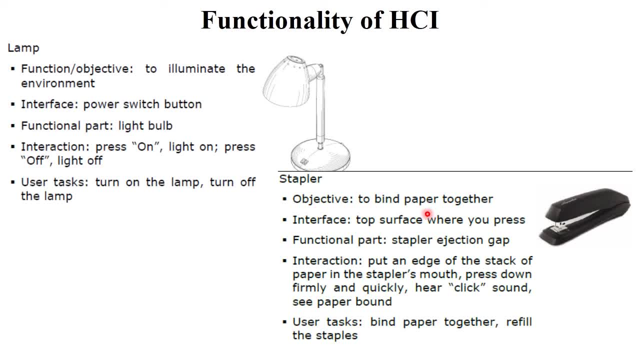 Ok. The objective of stapler is to bind the paper together. Interface is top surface. where you press The functional part is stapler. ejection gap: Ok. And interaction Put an edge of the stack of the paper in the stapler's mouth. Press down firmly and quickly. 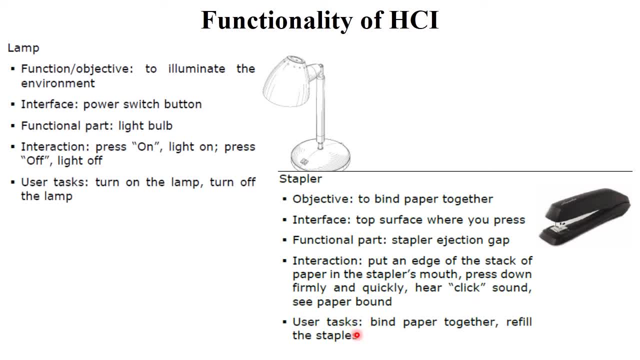 Here, click sound, see paper bound. And user task is: bind paper together, Refill the staples. Clear, So stapler is also easy to use. Each and every generation's people use this types of product. Clear So there are concepts And their development is more easy. Clear, Ok Next. 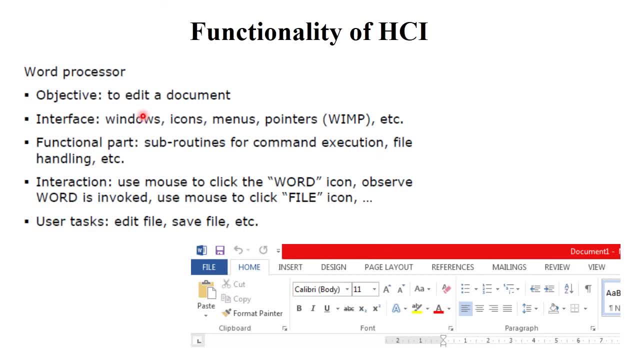 Next example of functionality is word processor. We all are familiar with Microsoft word. Ok, In my previous video We already told about. I only told about Microsoft word goals. Ok, You have to refer this Clear. So objective of word processor is to edit a document. Right Interface is windows.